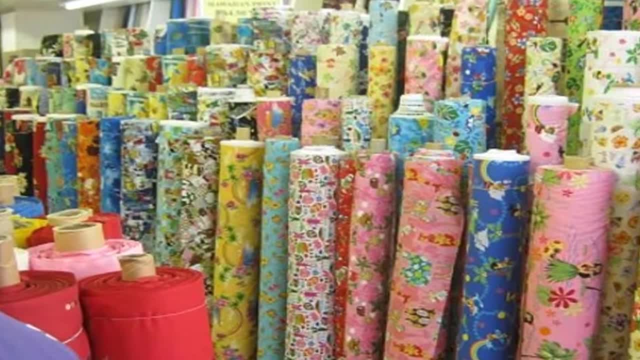 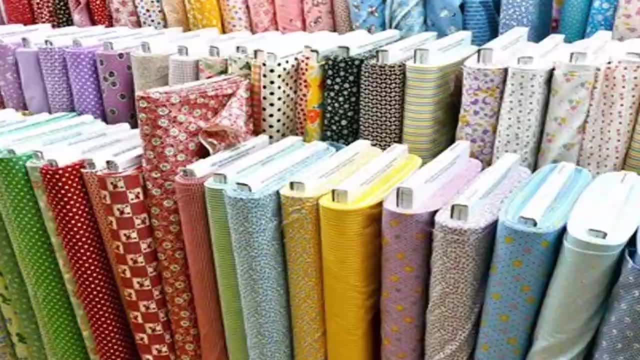 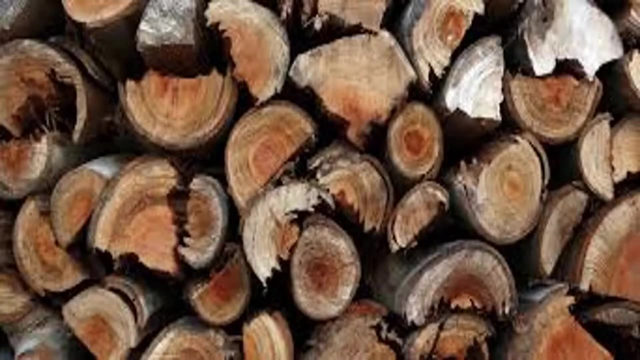 Plants are the largest providers of textile and fabric material. These materials are eco-friendly, compatible and less expensive, So they are used for making cloth, which is required by humans. The plant wood is used to build houses and also to make furniture items like chairs. 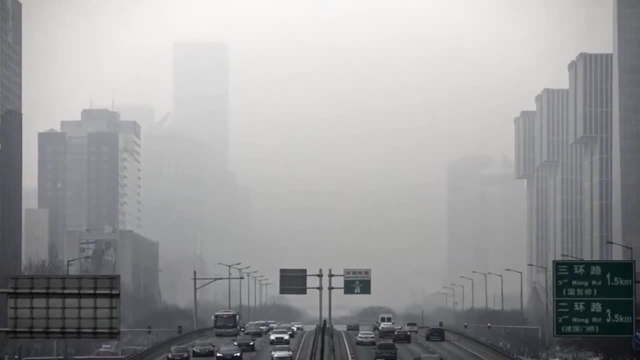 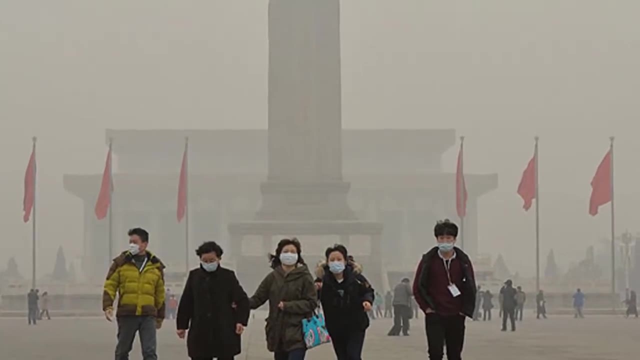 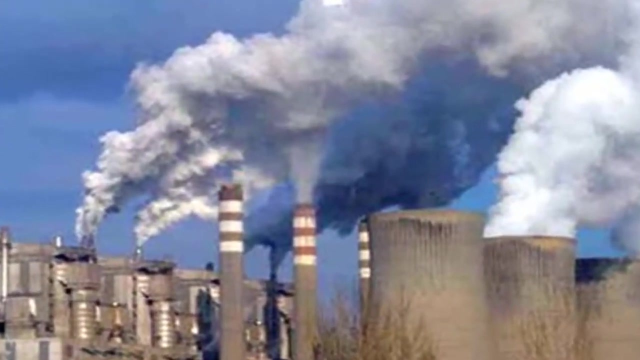 shelves, tables, etc. In cities and towns there is a rise in air pollution, So city environments are highly polluted and unsafe for living. This is due to automobiles and factories ejecting toxic gases and reducing the healthy oxygen ratio of air, So growing plants on earth will increase oxygen production. Thus the health of plants will be reduced. Plants are killed off by air from the time they are known. This means that the amount of oxygen in air is reduced, so the health of plants goes up. So growing plants on earth is the same as the health of plants in other countries. These activities are required to protect our environment. 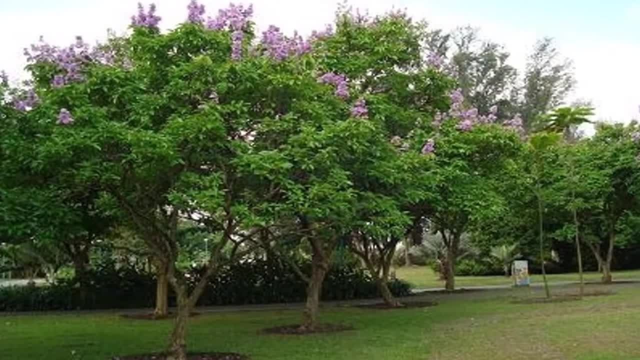 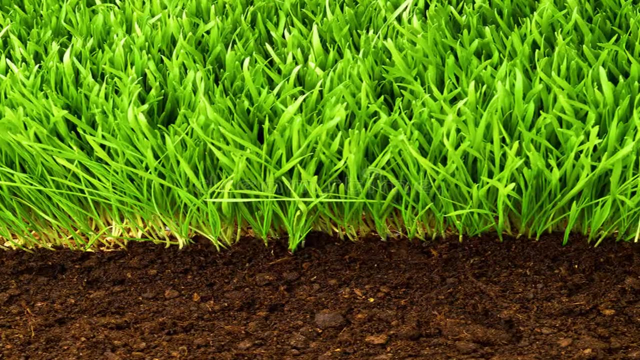 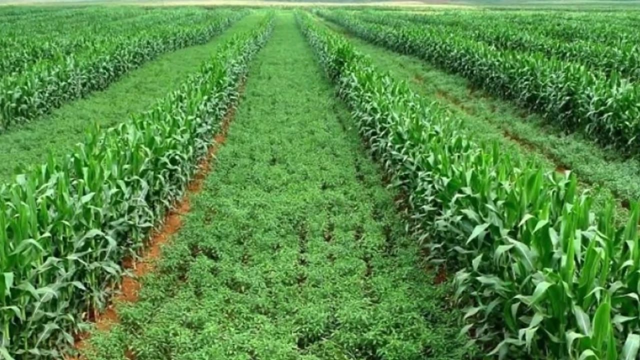 So growing plants on the roadside, parks etc. helps minimize the air pollution. Plants, when grown in dense, prevent soil erosion. In times of winds the fertile top layer of soil is carried away by air. This is prevented by plants if grown around. 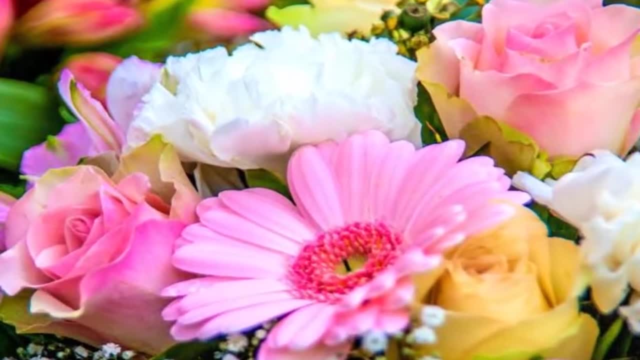 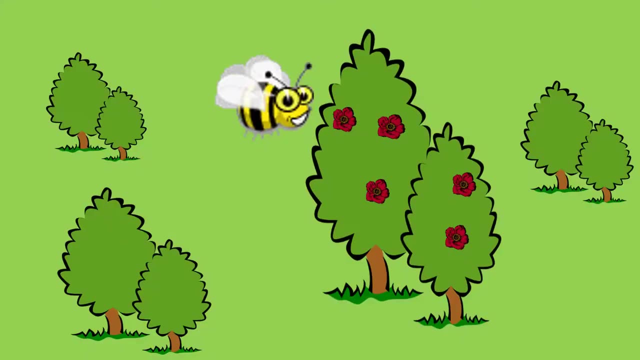 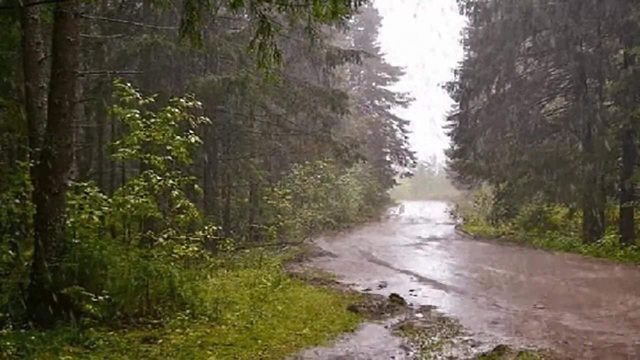 Flowers are used widely by humans. Flowers are also used to produce fragrance, and even their scent is extracted for daily use From flowers. the bees produce honey. Plants and trees have a cooling effect on the atmosphere, leading to rainfall. 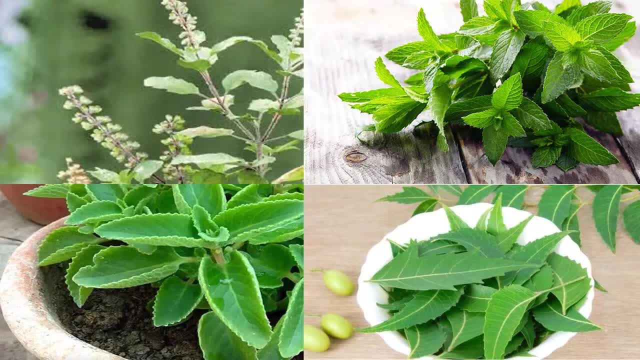 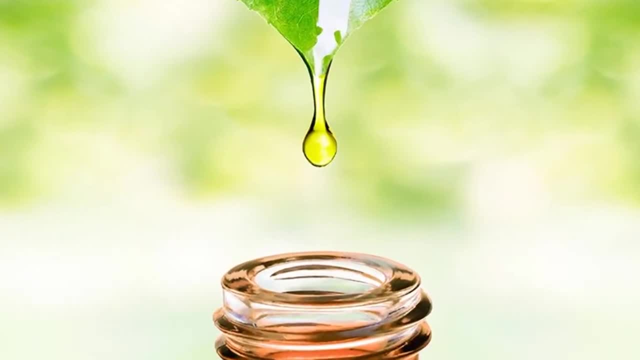 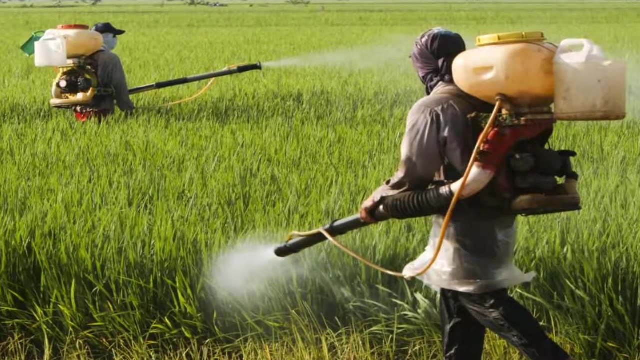 Plants are an excellent source of medicine. Plant medicine is safer due to their lower chances of side effects. Plants are also the source of insecticide. Plants are also the source of pesticides, and pesticides Using artificial pesticides are harmful to the environment. 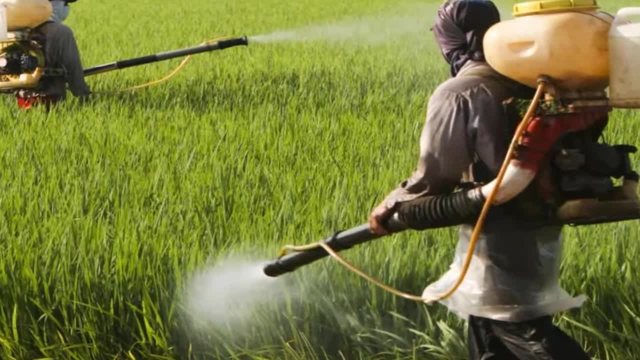 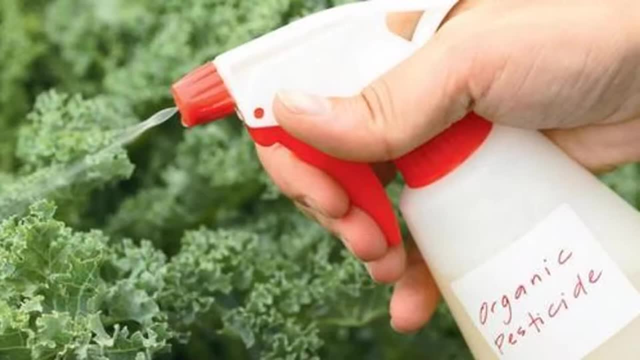 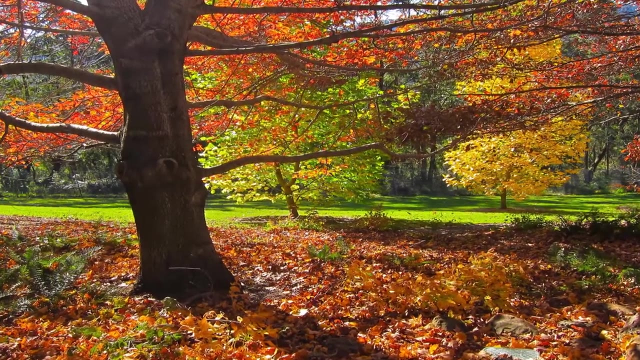 They may even enter food, causing health issue to human and animals. Using naturally derived pesticides are safe. Plants maintain soil fertility. Their droppings and shedding of leaves, fruits and other parts degrade in the soil to form humus. 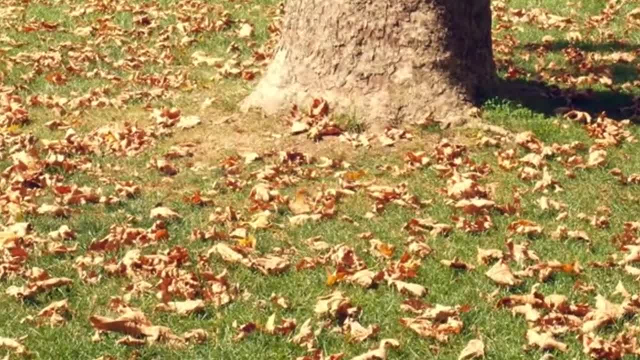 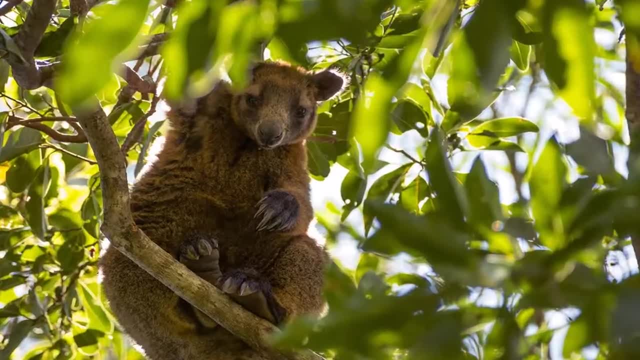 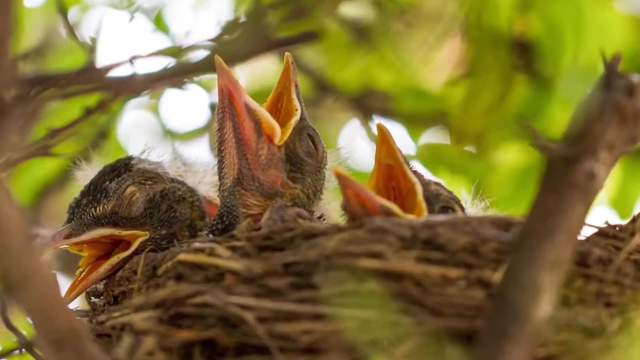 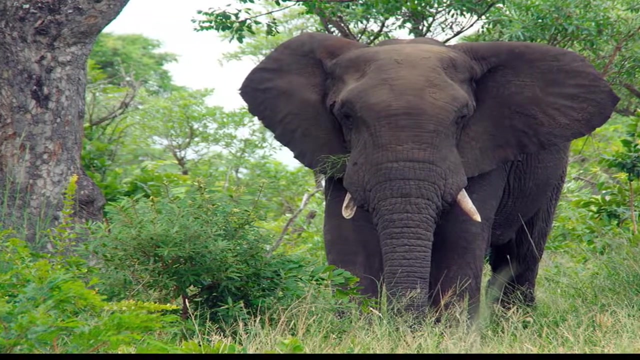 This humus increases soil fertility. Trees are the best places of shelter for birds and few animals to live. Birds build their nests for hatching eggs, sleep, hunt and safety on the trees In forests. animals can take shelter under trees in heavy summers and rain.